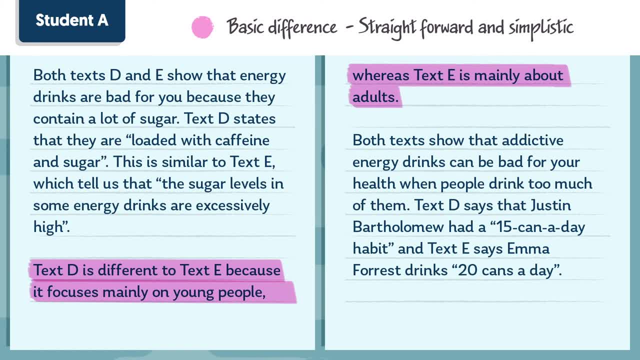 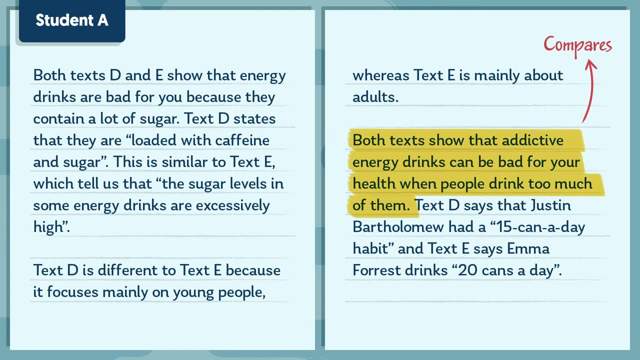 but this point is rather straightforward and simplistic. They also haven't used any quotations to back it up. In their final point here, Student A compares what's said about the addictive nature of energy drinks and does use a suitable quotation to support their points. 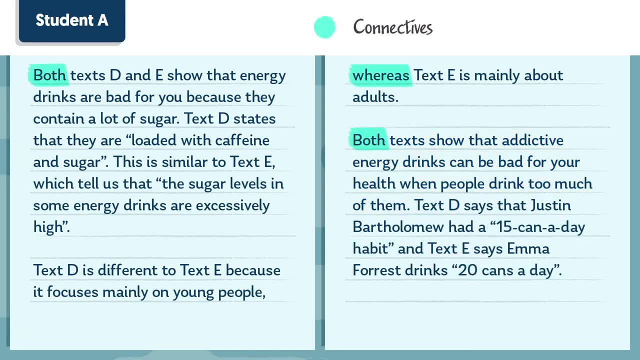 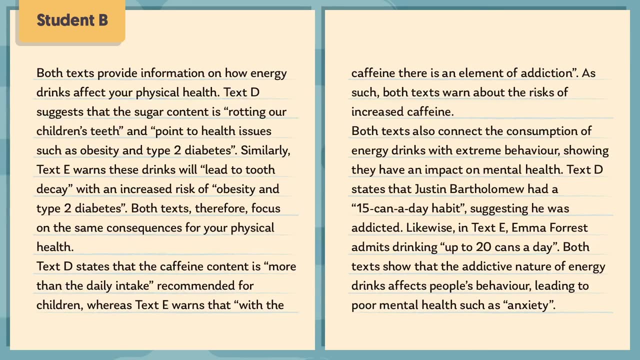 They clearly identify the texts and use connectives, like both and, whereas appropriately, but they don't fully explain their ideas. So Student A would receive between 5 and 6 marks if they continued their answer in this way. Now let's move on to an extract from Student B's answer. 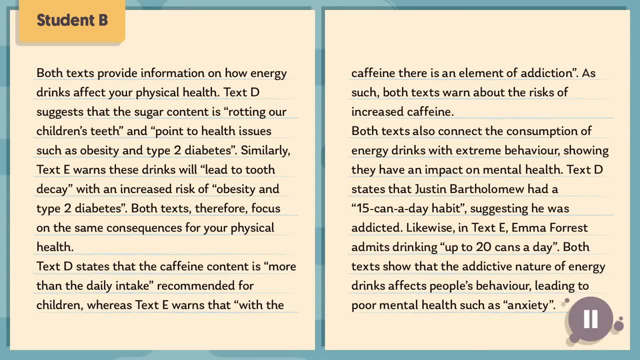 Press pause now to give yourself time to read it through and press play again when you're ready. Like Student A, this student uses quotations from the two texts in their answer to support their ideas about similarities and differences, but they then go an extra step and clearly explain what the similarity or difference is. 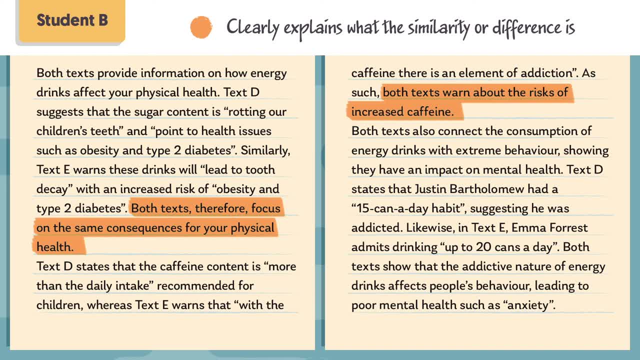 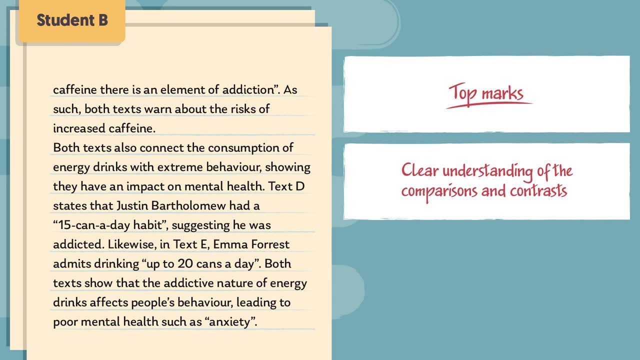 For example, in addressing how the texts present the impact of energy drinks on physical health, the student says: Both texts warn us about the effects of energy drinks on physical health, but they also warn us about the effects of caffeine. This is a key requirement because for top marks the examiner needs to see that you have a clear understanding. 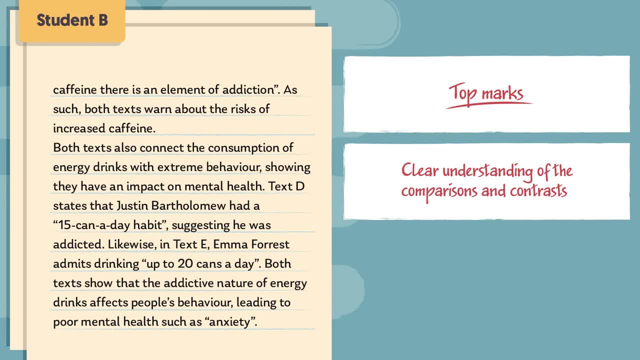 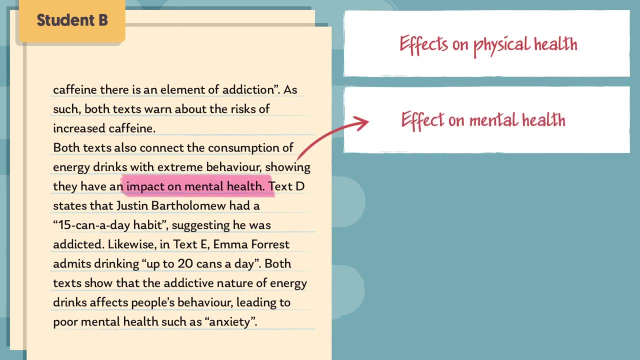 of the comparisons and contrast between the texts, As well as the clearer explanations. the best thing about this student's answer is that they address a wider range of aspects of the topic. As well as comparing the effects mentioned on physical health, they also make comparisons about the effects of energy drinks on mental health. 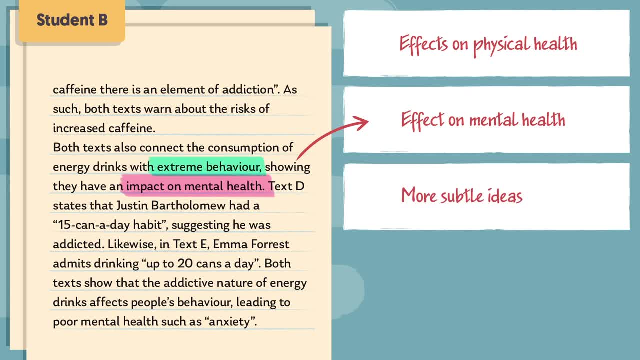 looking for more subtle ideas and explaining how. both texts show that energy drinks can lead to extreme behaviour. This is a more sophisticated approach and helps the student earn marks in the highest band. Their answer is really thorough, meeting the examiner's requirements for top band answers to be sustained and detailed. 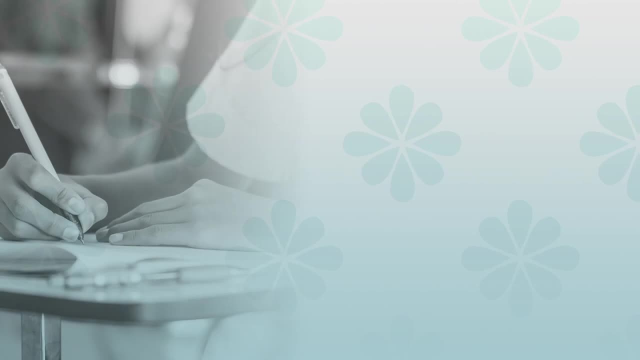 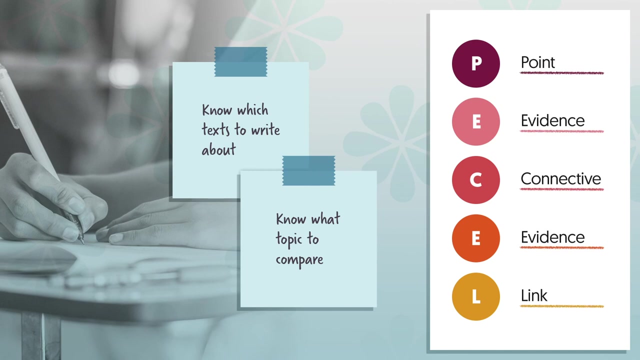 We'll leave it there. So, to be successful on this type of question, remember our top tips for comparison, Know which text to write about, Know what topic to compare, And remember to PEC-EL Point Evidence- Connective Evidence Link. 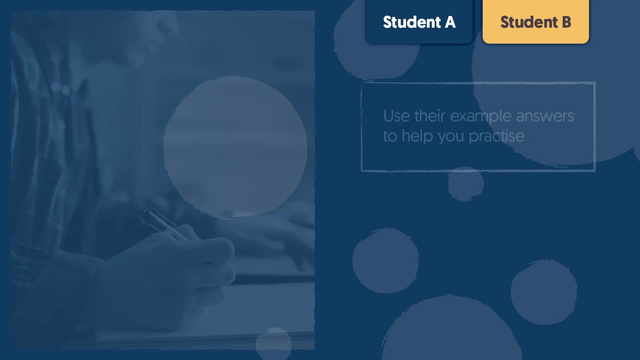 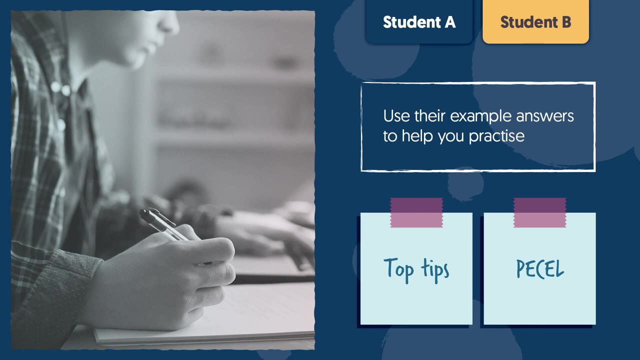 Now you know how these candidates achieve their marks, why not use their example answers to help you practice some comparison questions of your own. Use our top tips and suggested structure to guide you. Good luck.